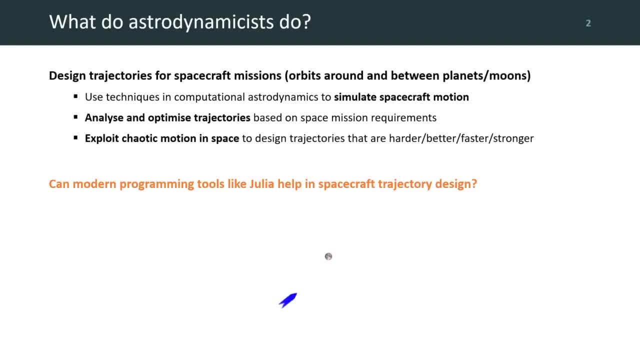 so can modern programming tools like Julia help in spacecraft trajectory design? Well, yes, we can help improve development efficiency and computational performance. We can provide access to state-of-the-art methods and perhaps inspire and enable novel approaches in astrodynamics. So to demonstrate this, 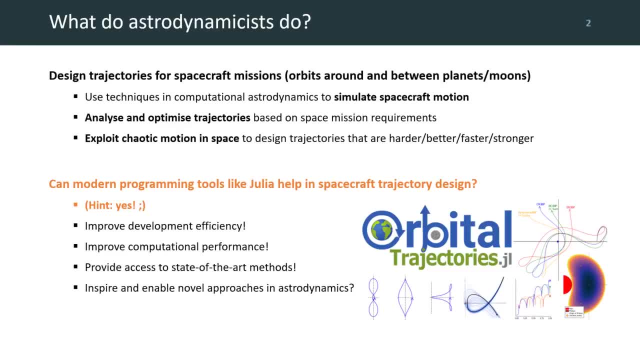 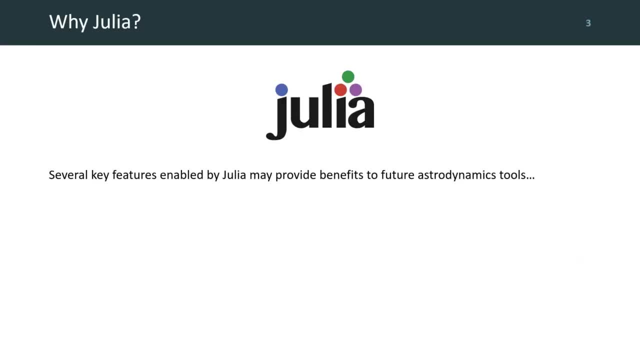 I've been developing orbitaltrajectoriesjl, a proof of concept package for spacecraft trajectory design in Julia. But why should we use Julia? Well, if you're watching this talk, then you probably already know about a few of the things that make Julia a particularly attractive. 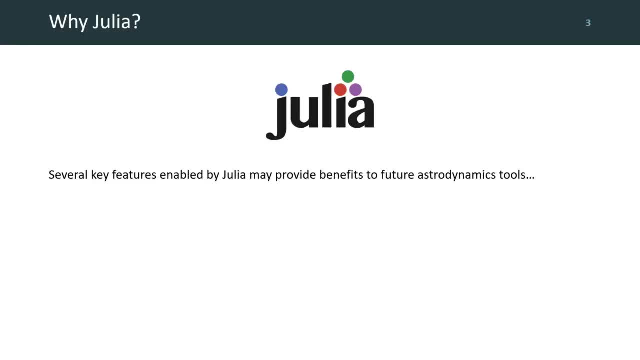 tool. We've heard of several key features enabled by Julia, which we believe may also provide benefits to future astrodynamics tools. Namely, Julia is a modern, high-performance programming language that leads to state-of-the-art in differential systems, statistical analysis, machine learning and in other fields. It provides functionality for 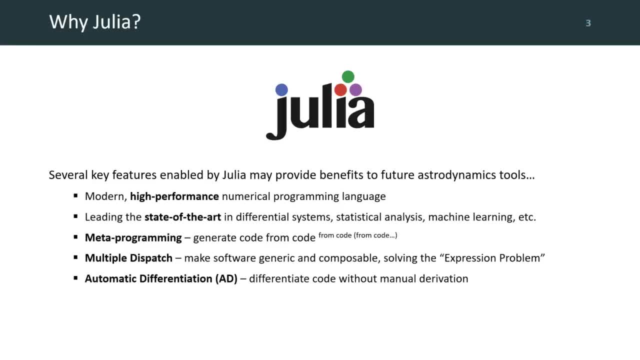 metaprogramming, which allows you to generate and manipulate code from code itself. multiple dispatch, which helps make software generic and more composable by making it easier to express new types and functionality, and allows for almost universally differentiable code providing accurate. 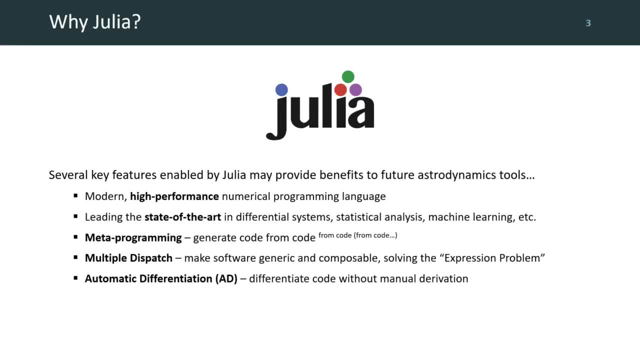 differentiation without resorting to approximations or analytical derivatives. Individually, these techniques are already used in many applications in and outside of astrodynamics and other fields, but combined they may lead to more efficient and possibly innovative new methods and tools. Let me give you an example of how we can. 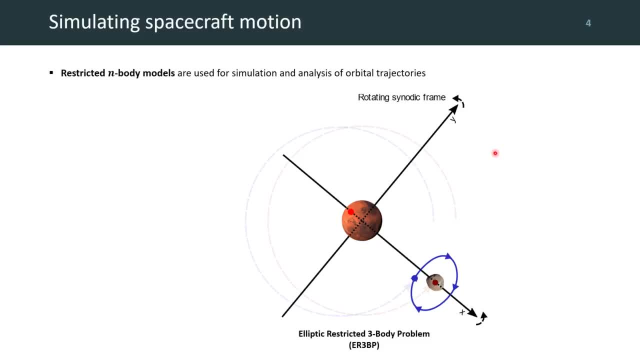 simulate spacecraft motion using a so-called restricted n-body model. Here we have a system that is restricted to three bodies: Mars, its moon, Phobos, which orbits in an ellipse, and a spacecraft. The equations of motion for the spacecraft are defined by this set of second-order. 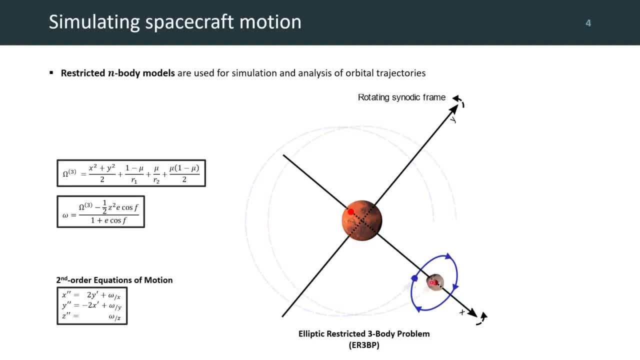 differential equations which essentially define the acceleration of the spacecraft as a function of the rotating frame of reference which follows the moon Phobos, plus the gravitational attraction both to Mars and to the much smaller moon. Developing simulations for this system generally requires hand-deriving and hand-coding derivatives of these functions. Instead, using the modeling, 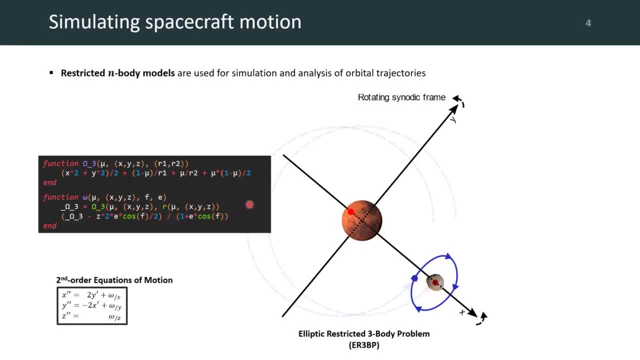 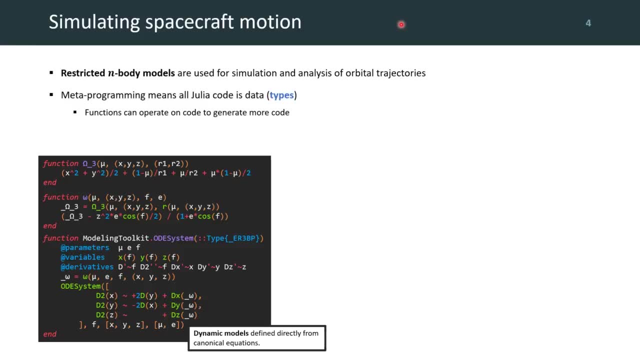 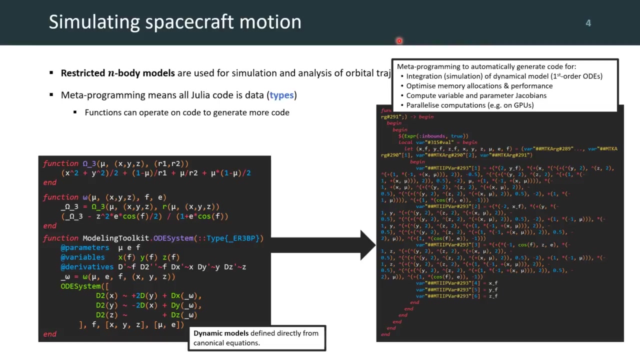 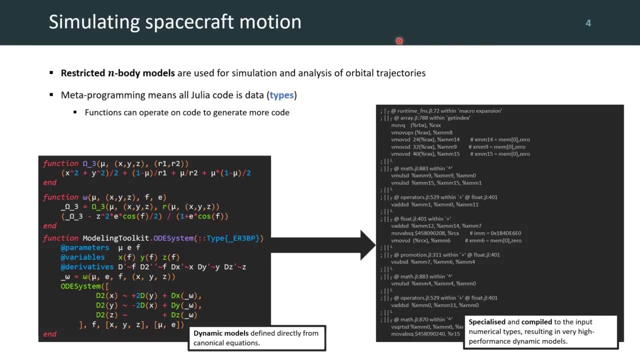 toolkitjl package, we can simply define these as functions directly, then define symbolic variables and parameters that stand in for the numerical values, allowing us to directly represent the equations of motion of our spacecraft. So in the end, without having to hand-derive or hand-code it, we have a 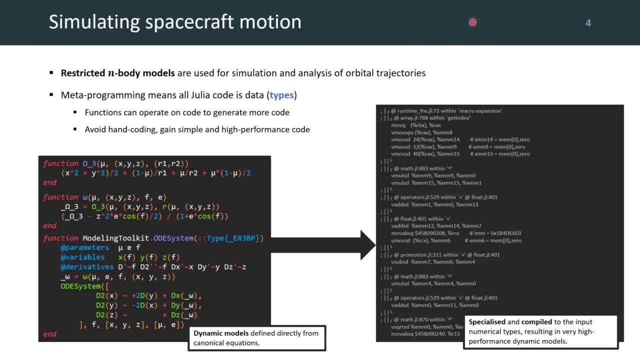 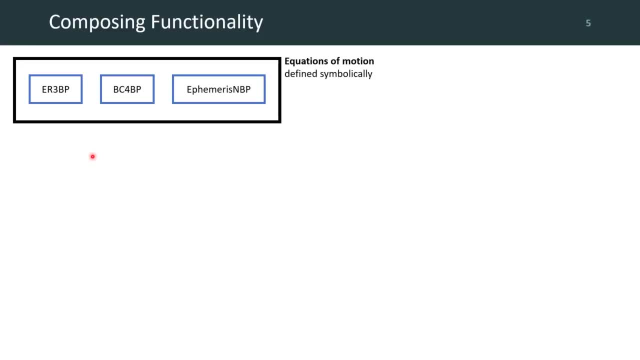 simple and extensible definition of our model that still provides extremely high performance execution. Using such techniques, I've been able to define symbolic equations of motion for various astrodynamical models, including the elliptic restricted three-body problem, the bicircular restricted four-body problem and the ephemeris restricted n-body problem. Now, through 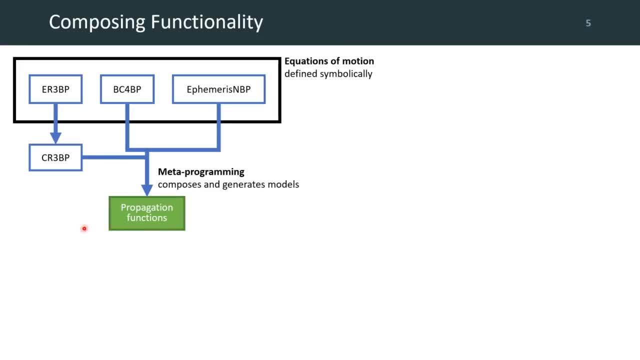 metaprogramming, we can automatically generate not only the propagation functions, as I showed before, but we can also generate new models directly from the existing ones, such as the circular restricted three-body problem, which simply substitutes an eccentricity of zero into the 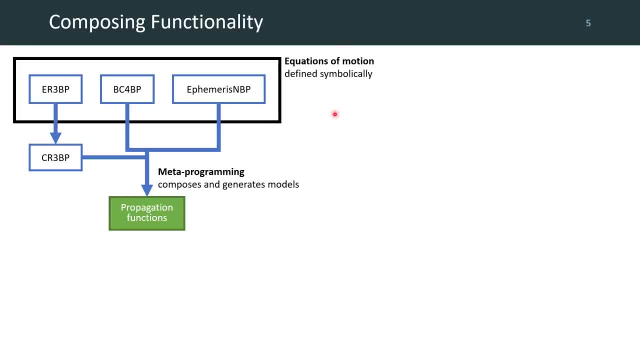 model. Currently I'm also experimenting with composition of models, together with custom perturbations such as solar radiation pressure. Now we can take these propagation functions and pass them directly to methods for generating and correcting trajectories. With Julia's multiple dispatch feature, these methods are made generic, effectively accepting. 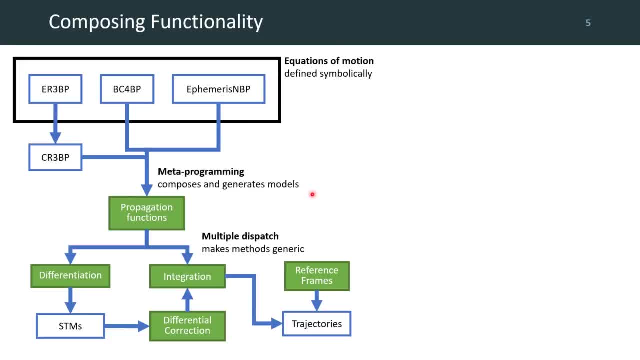 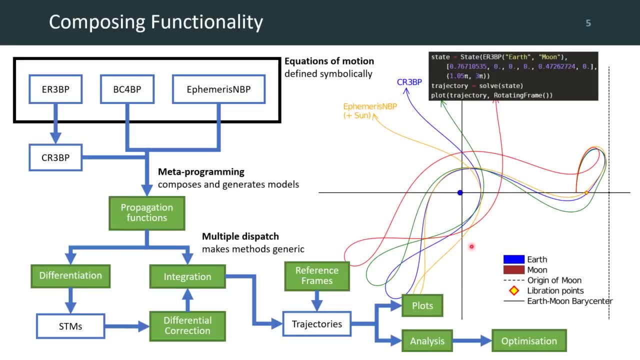 any of the four models, while still being specialized by the Julia compiler to provide high-performance computation, And this extends to functionalities such as plotting and analysis of trajectories as well. So, for example, we can easily simulate and plot trajectories by passing in a different model, a different initial model and a new model. So, for example, we can easily 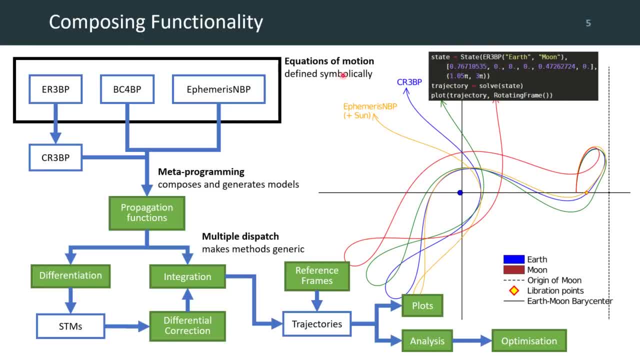 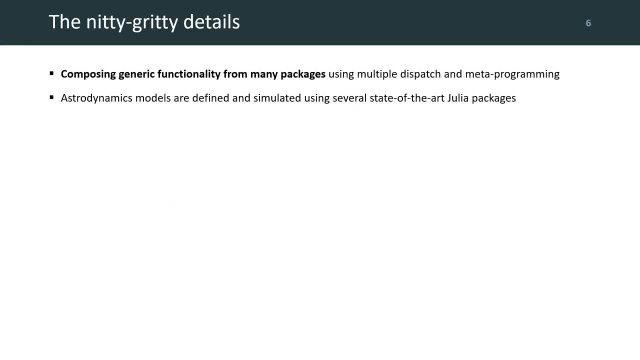 simulate and plot trajectories by passing in a different model, a different initial model and a new model. So what Julia gives us is the ability to compose generic functionality from many packages using multiple dispatch and metaprogramming. Our models are defined and simulated using several state-of-the-art packages, including, again, modeling-toolkitjl. 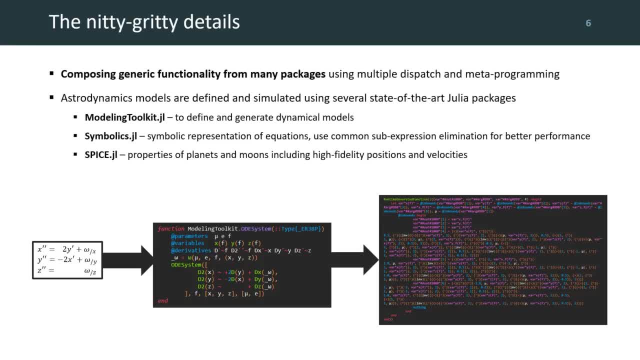 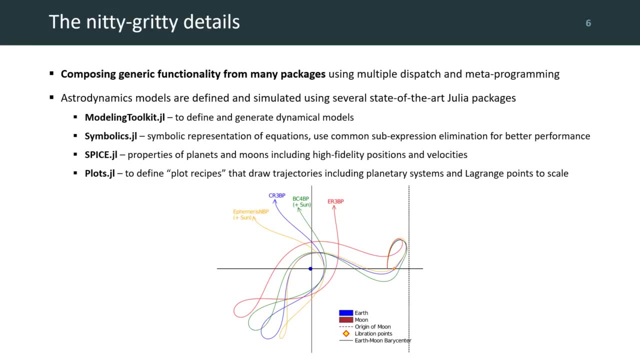 also symbolicsjl, which lets us manipulate the equations and use upcoming features like common sub-expression elimination to provide better performance. spicejl to access high fidelity positions and velocities of planets and moons. plotsjl to define plot recipes that draw trajectories including planets, moons and Lagrangian liberation points to scale. 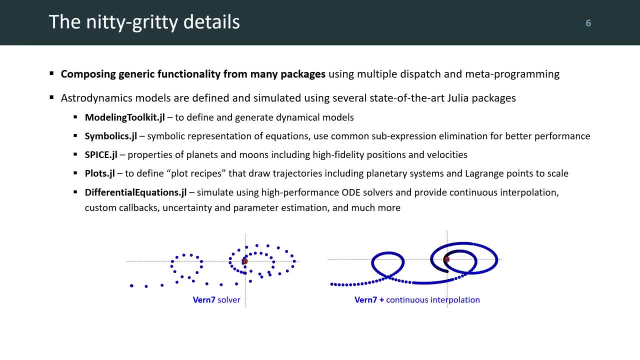 and, most importantly, differentialequationsjl, a cutting-edge package that allows us to simulate the spacecraft trajectories using any one of dozens of high-performance ODE solvers, with support for high-order interpolation, custom callbacks, uncertainty and parameter estimation, and much. 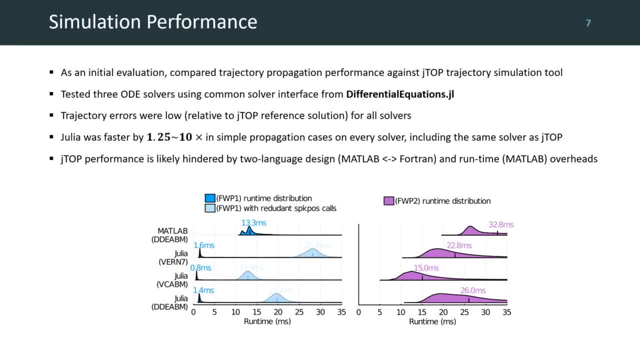 more. I compared the performance of my automatically generated simulators against an in-house astrodynamics tool at JAXA called JTOP, which has a Fortran core for simulation sitting behind a user-level MATLAB library. Now, not only do we have the ability to simulate and plot trajectories, 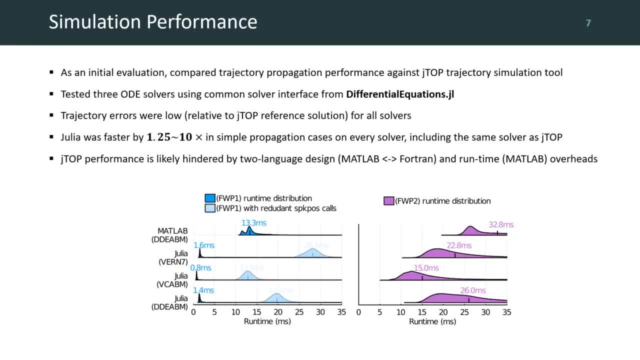 but we also have the ability to simulate and plot trajectories using any one of dozens of high-performance ODE solvers with support for high-order interpolation, custom callbacks, uncertainty and parameter estimation. not only did all the Julia solvers provide highly accurate solutions compared to the reference. 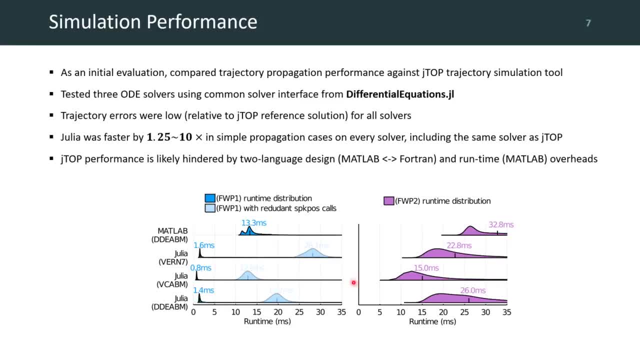 trajectories. they were also computed up to 10 times faster in every case, even when comparing with the same solver used by JTOP. This massive performance benefit is probably because Julia avoids the overheads of a two-language design. An important part of trajectory design is the 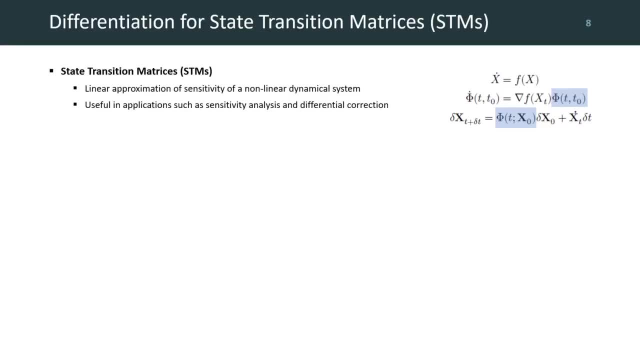 computation of State Transition Matrices, or STMs, which are a linear approximation of the non-linear dynamics of the system and are used for applications such as sensitivity analysis and differential correction. I tested four ways to calculate the performance of these systems. I tested four ways to compute these in Julia, The hand-coded way in which we manually derive the 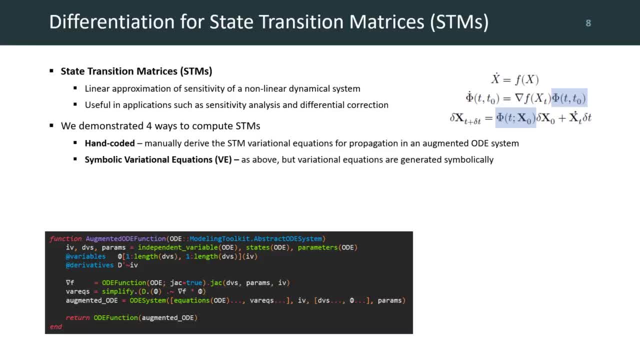 equations necessary and include them directly in an augmented ODE system. Symbolic variational equations in which we use modelingtoolkitjl and symbolixjl to automatically derive and compose, together with the existing symbolic models, Finite differences, in which we simply propagate the 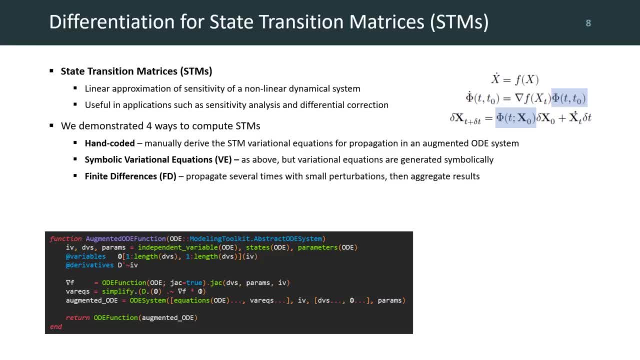 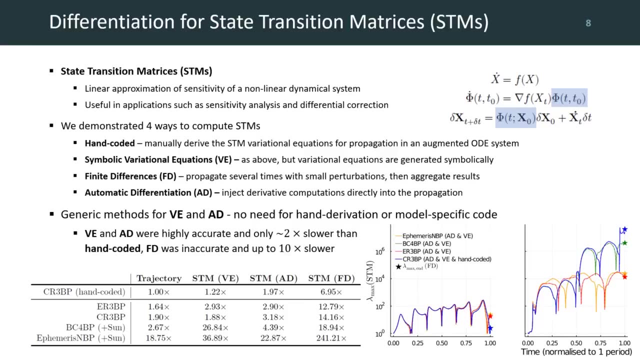 trajectories multiple times with small perturbations and then aggregate the resulting differences And automatic differentiation, in which we inject so-called dual numbers directly into the propagation. These compute their own derivatives at the same time as the simulation, requiring no other code. Both the symbolic and automatic differentiation methods are generic. 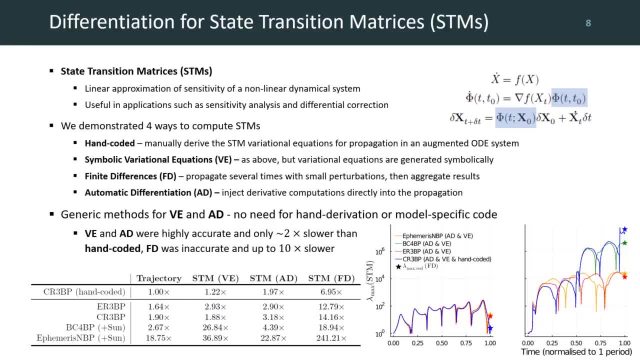 so they support any of the four models that we defined. They were found to be only two times slower than a hand-coded approach, which was only available for the simplest model, as well as greatly outperforming the finite differences method in both speed and accuracy. 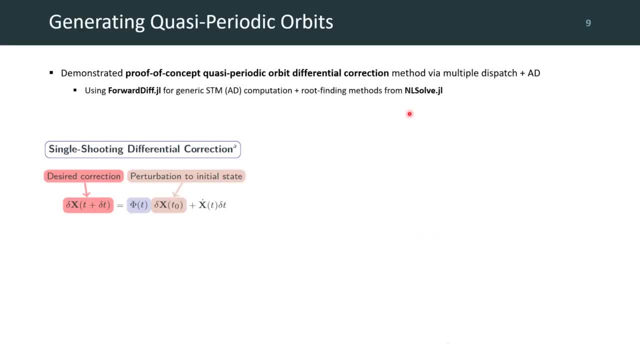 Using forwarddiffjl to provide automatic differentiation for my models, as well as root-finding methods from nlsolvejl. I also demonstrated a method for generating quasi-periodic orbits via single-shooting differential correction approach. Essentially, starting from an initial guess, we can target some sort of periodicity condition. 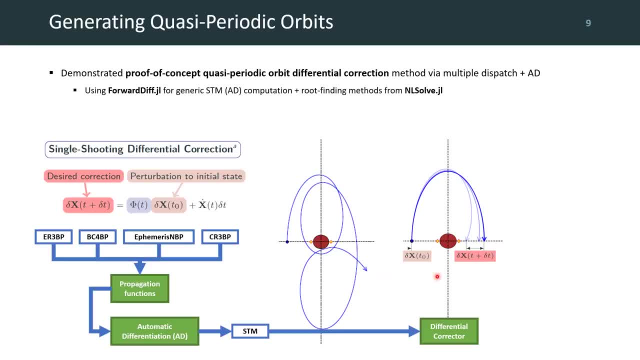 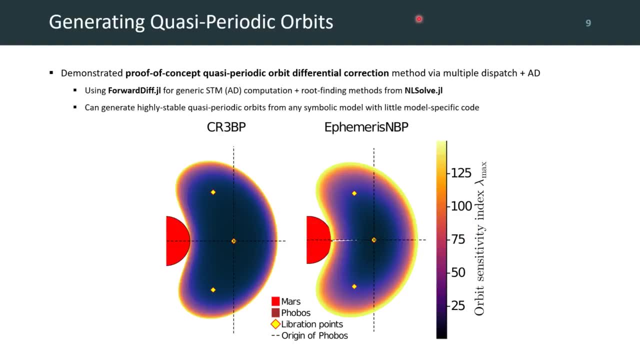 such as ensuring a perpendicular axis crossing, and correct our initial guess based on the remaining distance. Again, because Julia code can be written in a highly generic manner, this functionality automatically supports all of our models, allowing us to find families of periodic orbits, both in simple models like the circular three-body problem.